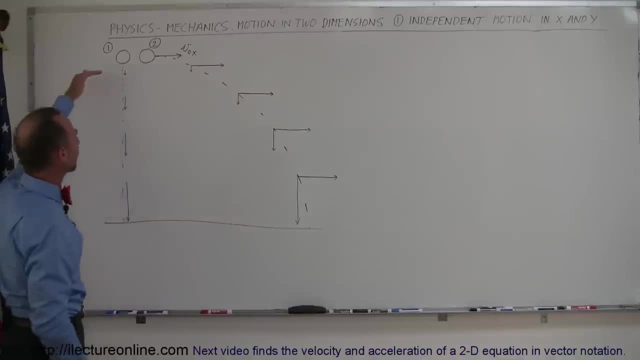 that seems a little puzzling because, intuitively, we would think that this ball, which travels a greater distance, would take longer to hit the ground before the ball that just gets you know drops straight down. And the reason why that is not the case, the reason why they hit the ground. 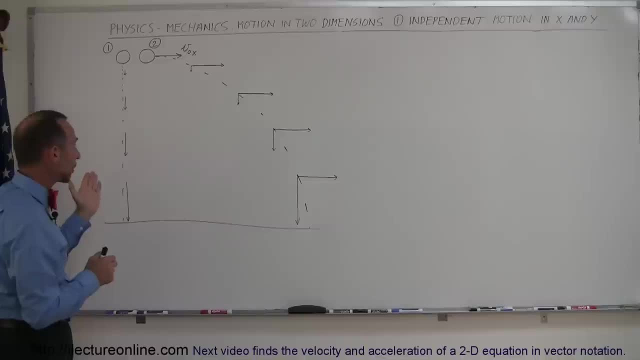 at the very same time is because the motion in the x direction and the motion in the y direction, so the horizontal motion of the ball and the vertical motion of the ball are completely independent of one another. Notice, in the horizontal direction there's no forces acting on the balls, so this ball will stay stationary in the x direction, simply fall. 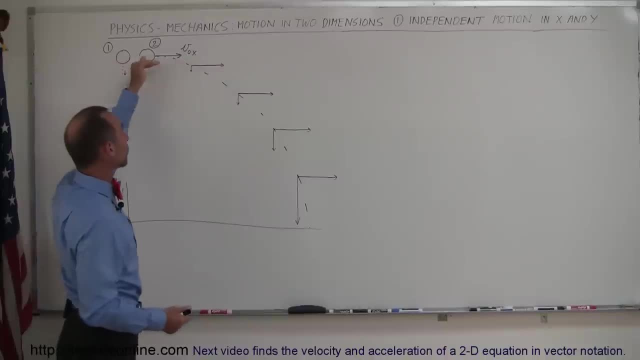 down in the y direction. This ball, once thrown out to the right at some initial velocity in the x direction, it will no longer feel a force in the x direction, and so the ball will simply maintain the same velocity in the horizontal direction, In the vertical direction, the y direction. 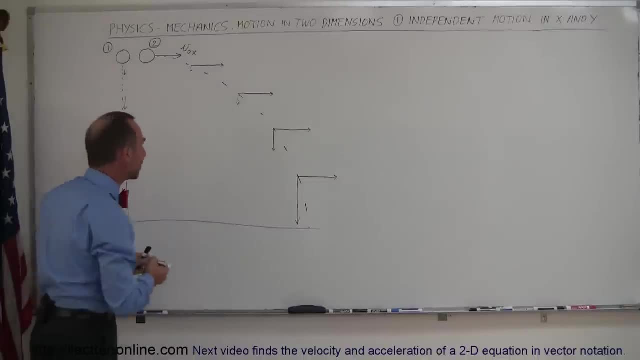 both balls will stay stationary. in the x direction, In the horizontal direction, both balls feel the exact same force. they feel the force of gravity. So on the left ball we have a force due to gravity and on the right side we have a force due to. 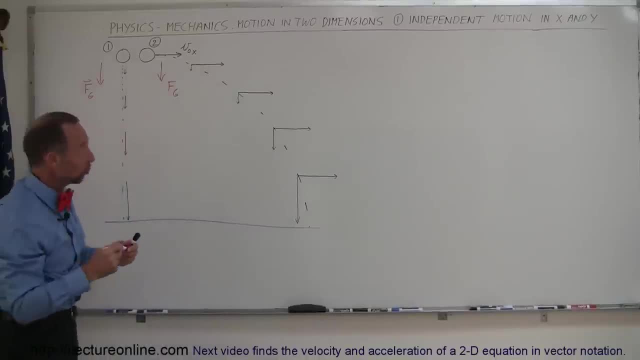 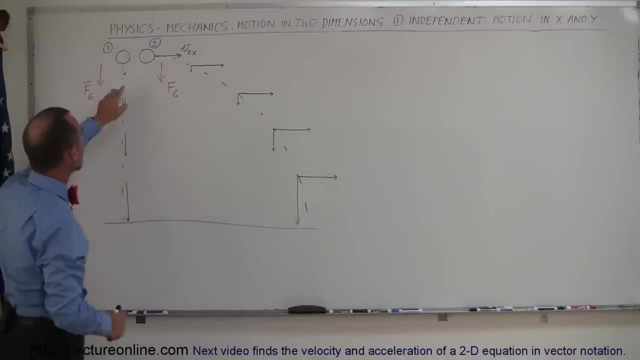 gravity. So both balls feel the exact same force, assuming that they have the same mass, and so therefore they're being pulled down or accelerated downward at the very same rate. You can see that the velocities in the y direction are the same at the same time interval, and you can see that. 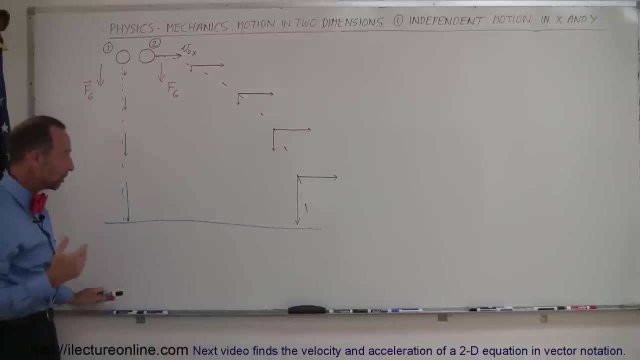 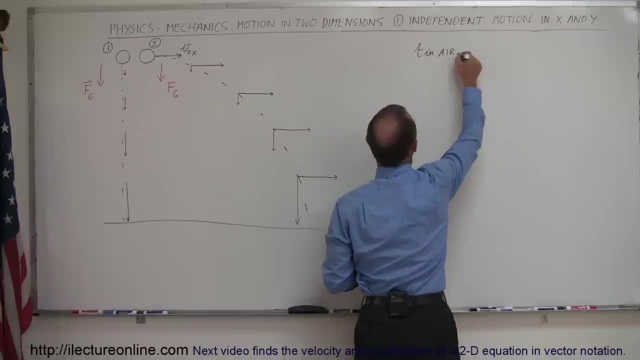 therefore, they will hit the ground at the very same time. So what can we learn from this? Well, first of all, we should learn that the time in the air for ball number one is equal to time in the air for ball number two. So that is really important. Later on, 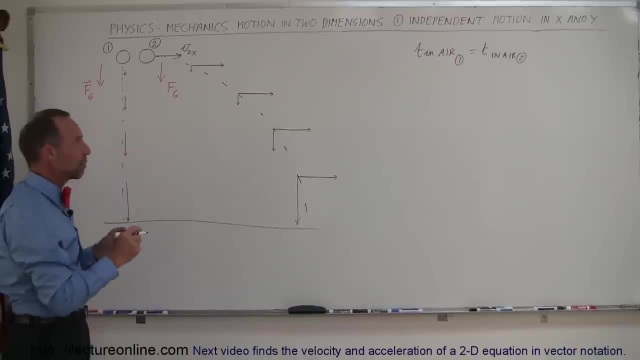 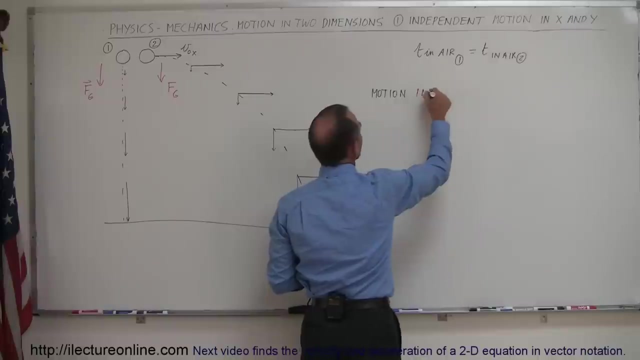 when we start doing problems and examples. that concept is extremely important. So the time in the air for any projectile, no matter what happens to it, only depends upon the vertical velocity and the vertical forces. Also, we should always keep in mind that the motion in the x direction, so we're talking about the horizontal direction. 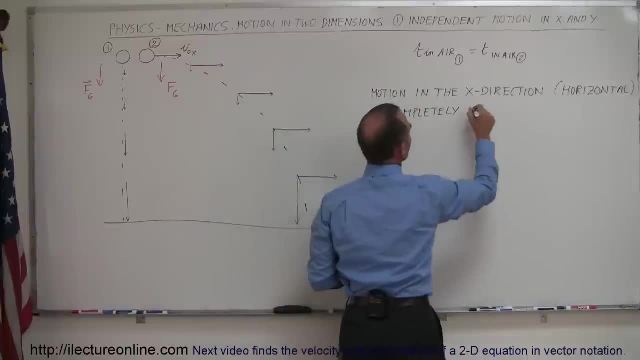 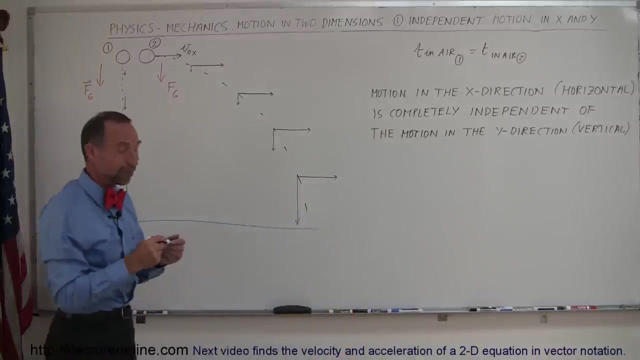 is completely- and I mean completely- independent of the motion in the y direction. Of course that would be the vertical motion. So why did I take the time to write that down? Well, it's a really important concept. So in all problems I'm going to do with projectile motion, you can look at the 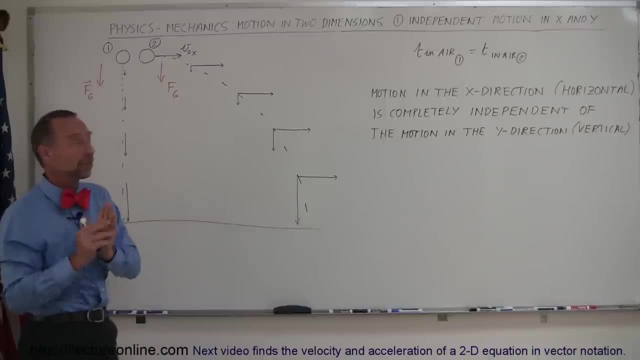 times of motion. andide sitzencn, and diagonal motion and vertical motion are completely independent, as they have nothing to do with each other. The only thing is that the time in the air depends upon how long it takes for the object to hit the ground in a vertical direction. 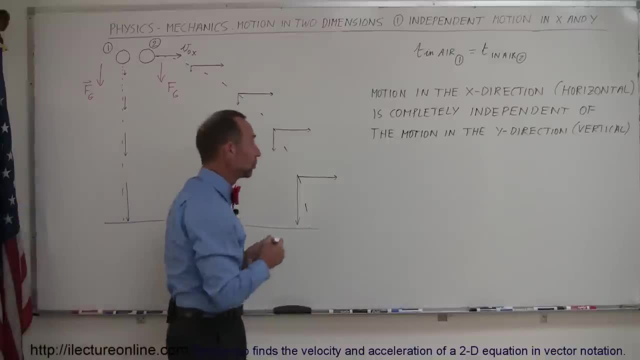 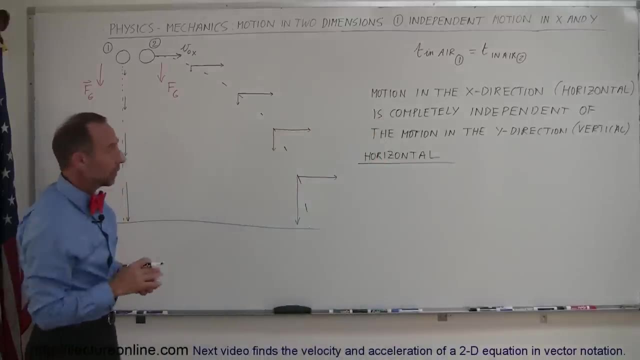 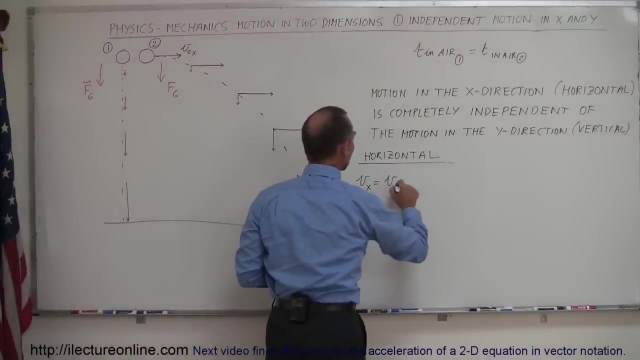 So let's now talk about how we describe the equations of motion in the two dimensions. So for the horizontal, since there are no forces acting on that in that direction, there's no gravity. in the horizontal direction, velocity in the x direction is simply equal to the initial velocity in the x direction. 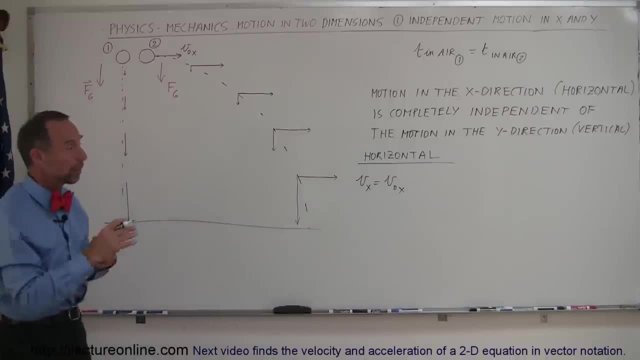 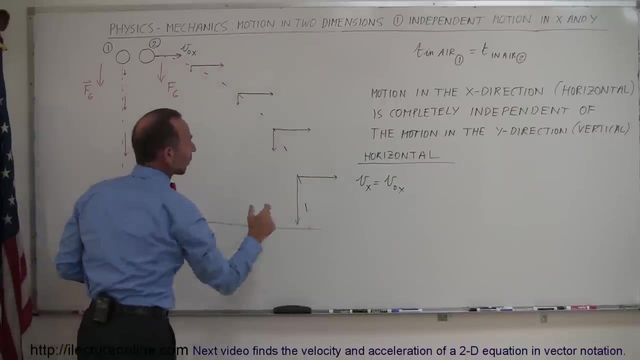 and it doesn't change. So whatever the initial velocity was in the x direction, it will maintain that velocity throughout its entire motion. It doesn't change. Notice that the arrow in the horizontal direction doesn't change. That represents velocity in the x direction. The 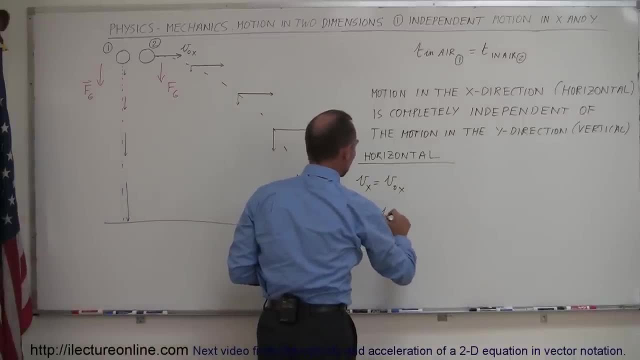 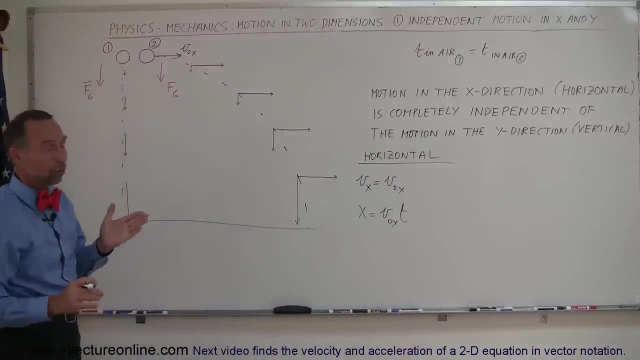 distance traveled in the x direction is simply equal to the initial velocity in the x direction times the amount of time that the object stays in the air, which is determined by the vertical motion. only Alright, On the vertical motion. the velocity in the y direction is equal to. 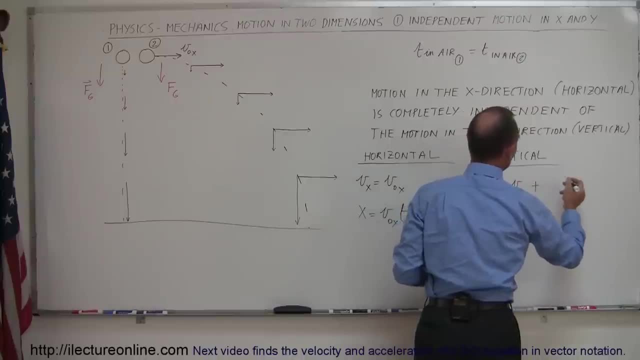 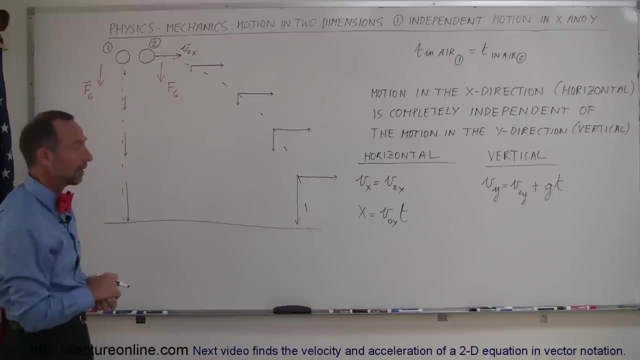 the initial velocity in the y direction plus the acceleration times time, and in this case we can probably just say that the acceleration for a projectile will be, of course, the acceleration due to gravity, and that's a minus 9.8 meters per second squared. Notice that, if it has, 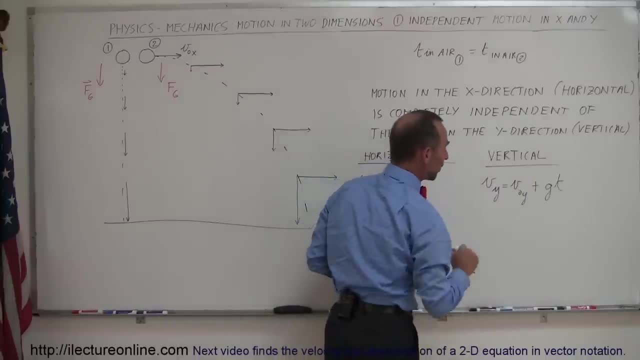 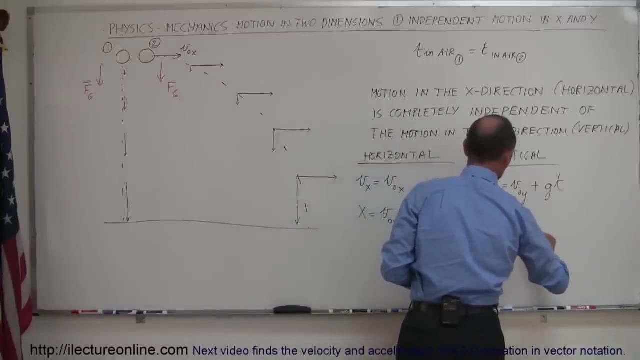 no initial velocity in the y direction, then v sub y is simply equal to g times t And for the position we can say that y is equal to t, The initial position in the y direction plus v, initial in the y direction times time plus. 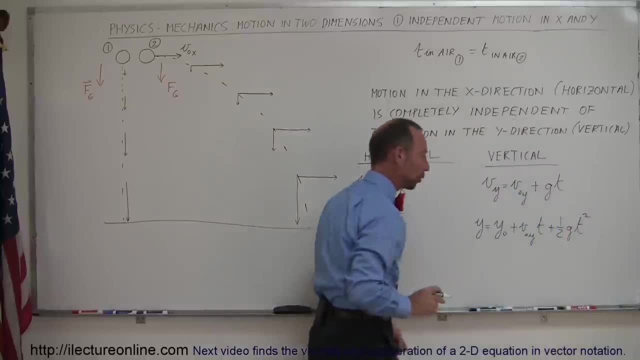 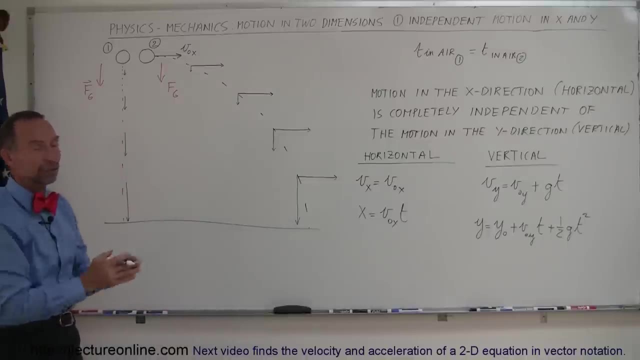 one half g t squared, and of course that came from the equations of motion. So those are the two ways in which we look at motion of a projectile, horizontally and vertically, and we keep them completely separate. So there's a nice little introduction of how to look.